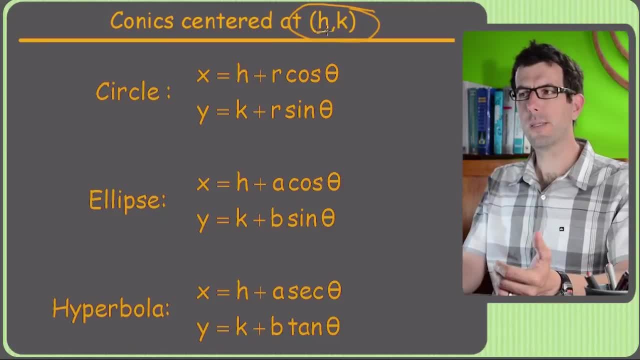 That's how you remember which one's h and which one's k. So the x coordinate is h, y coordinate is k, And that's why you're always going to see h's in the x equations and k's in the y's. 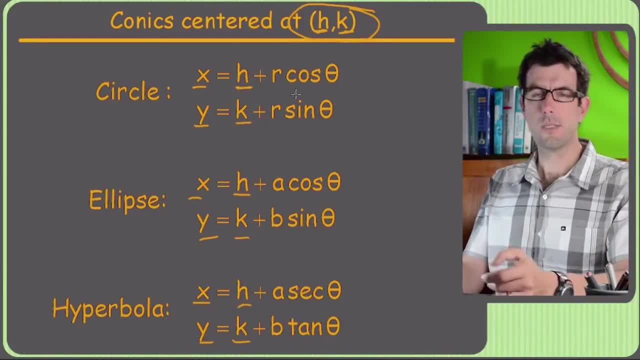 Alright. So that's the first thing to notice, Just like with the rectangular equations of ellipses, and circles. h and k just kind of get added in there in order to shift this thing up and around. The slight difference is that in the equation of a rectangular equation, a circle, 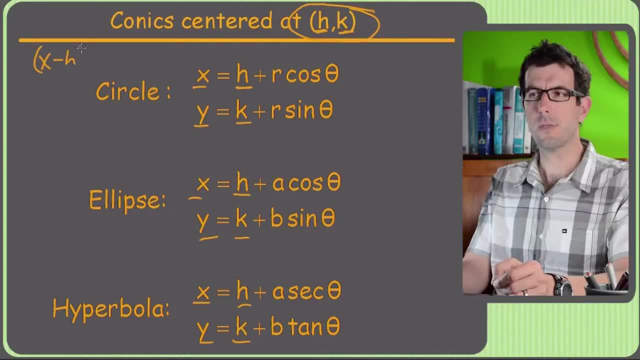 if a circle were entered, it would have an x minus h squared, And there was that. what I want to remind you of is that there's that h, x minus h right here. So if the center of a circle was at, x equals 2.. 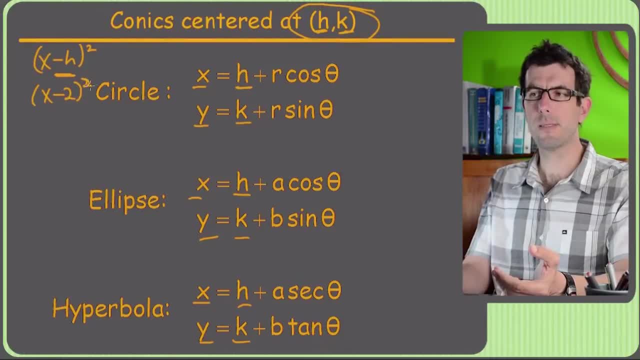 You're going to have x minus 2 squared in parentheses, because that's just the way it works. You do the opposite of the x coordinate, But in these equations there is no negative in front of the h, So that's just a little subtlety That actually makes these easier. 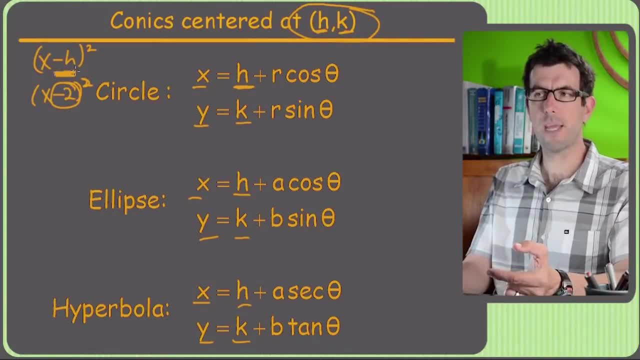 I just wanted to point it out so you don't get confused. In the rectangular versions we're going to have negative signs in front of the coordinates. basically take their opposites, But in their parametric equivalent we're just going to have a positive h and a positive. 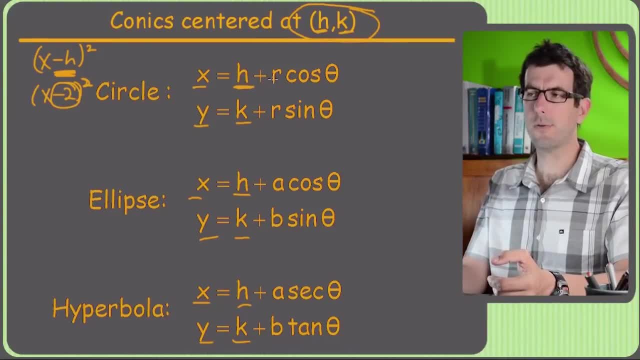 k. But other than that, if the thing is centered at 0,, 0,, for example, all the h's and k's go away, And you just end up with r cosine theta for x and r sine theta for y. Now what's? 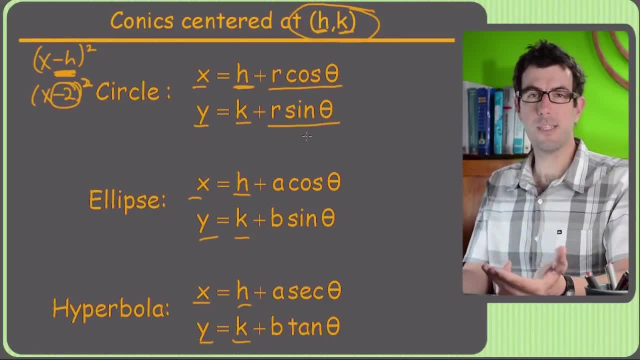 the difference between a circle and an ellipse. They're basically just the same thing. A circle is a special case of an ellipse where a and b are the major and minor axes. You might recall them being called in a previous class. The minor and major axis are identical in 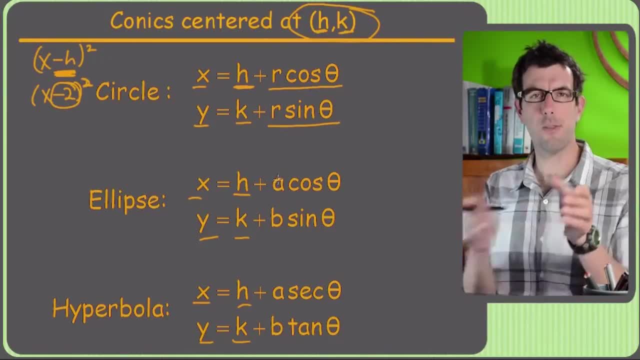 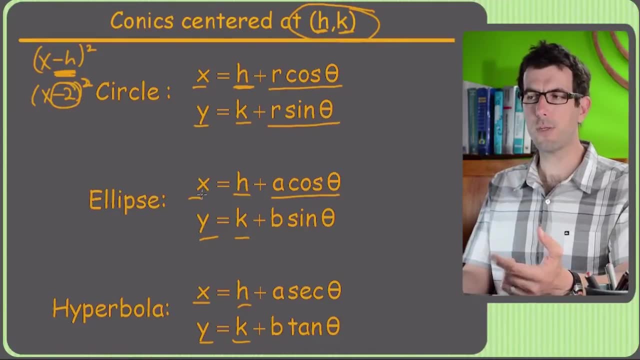 a circle, But in an ellipse, a and b are what they're called. So a and b are what they're called, basically the width and the height of the ellipse. And one subtlety is: I'm giving you the equations right here, and I have a on the x equation. 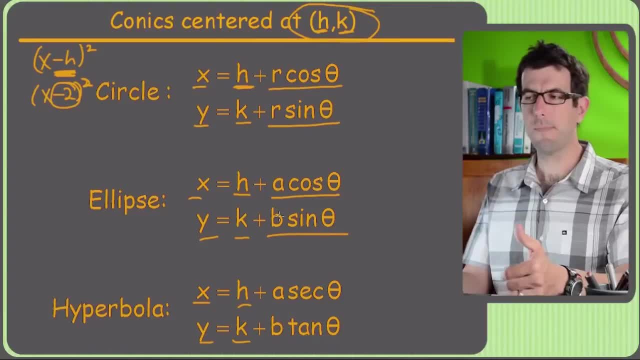 and b in the y equation. It doesn't matter, You can switch a and b, But the point is that whichever one of these coordinates has, the cosine is usually an x coordinate for an ellipse, And then the number in front of it just sort of tells you the width of the ellipse from. 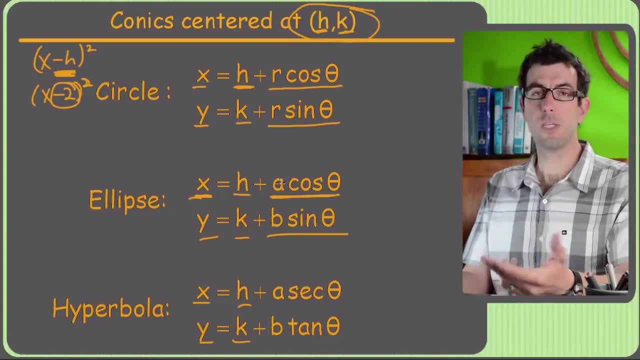 the center. So the width of the ellipse is actually going to be 2a, And then whatever's in front of the ellipse is going to be 2a, And then whatever's in front of the ellipse, whatever's in the y equation, like this b here in front of sine, that's going to be. 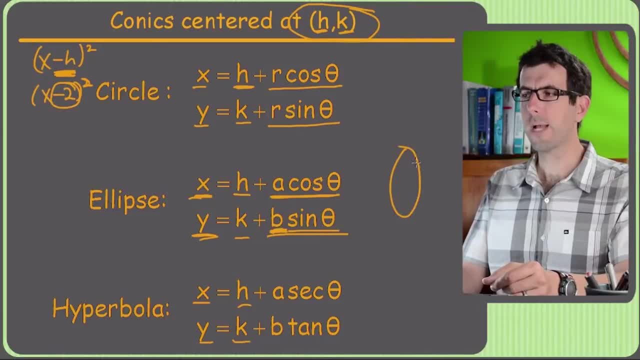 the height of the ellipse. And the overall height of the ellipse will actually be 2b And its width will be 2a, And that's just because a is actually the distance from here, from the center to the edge, And b is the height from the center to the top. So that's. 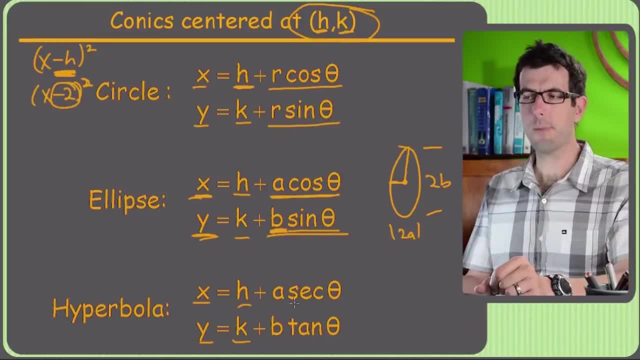 why the overall height would be 2a or 2b And hyperbola. very similar looking equation, except we switch cosine and sine out and put secant and tangent instead. Seems like a lot of classes don't cover hyperbola. 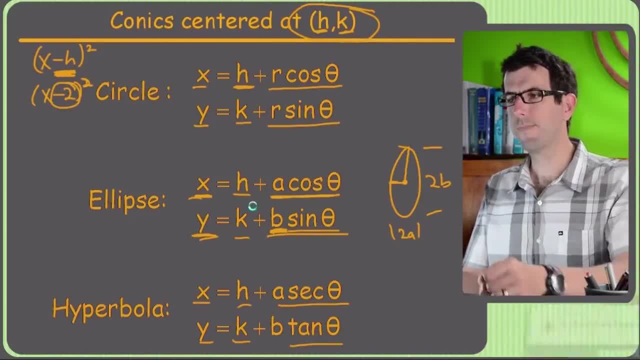 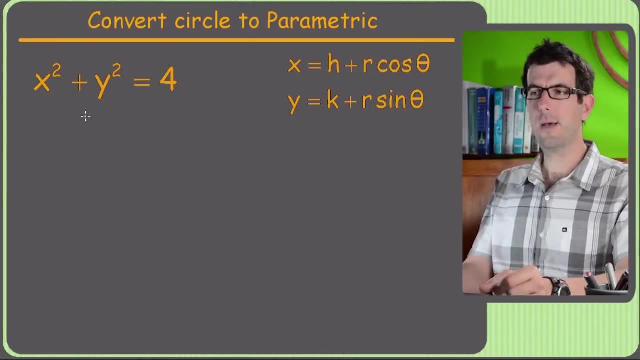 They're sort of pointless anyway. So all right, Let's take a look How do we convert this circle to parametric And, as I showed in the previous video, we could say: oh hey, you know, x equals t and therefore solve and get some crazy square root stuff. But I would 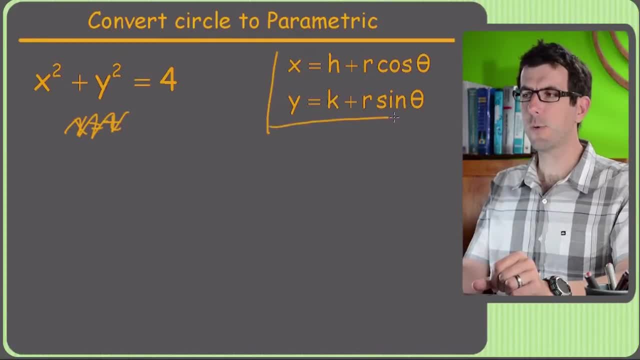 recommend just memorizing this. So I'm just. this is just here as a reminder for the generic equation of a circle. So just looking at this equation, because there's no parentheses, I know this is a circle centered at zero comma zero And I know it's right in the center. 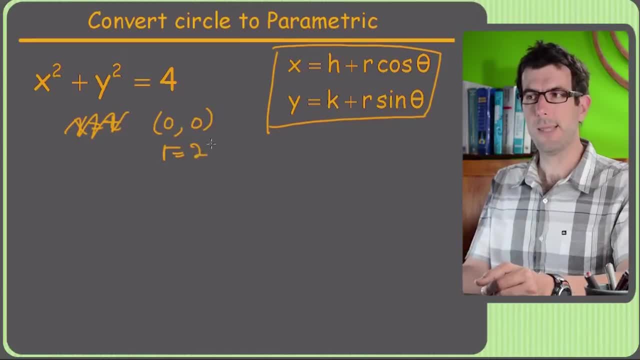 I know it's radius equals two. That's. the one way to screw these up is to not remember that the number over here is r squared, So you've got to take the square root to get the radius, And now we're just going to plug and chug. So x equals h, which is zero in. 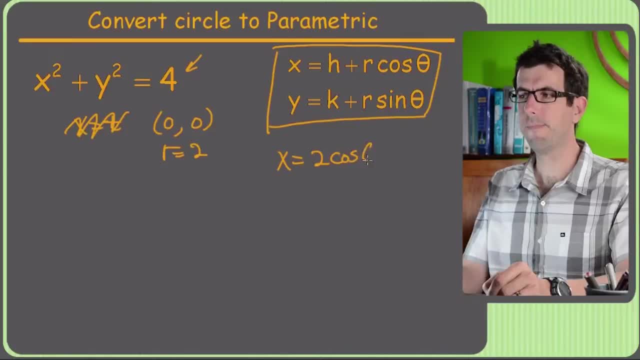 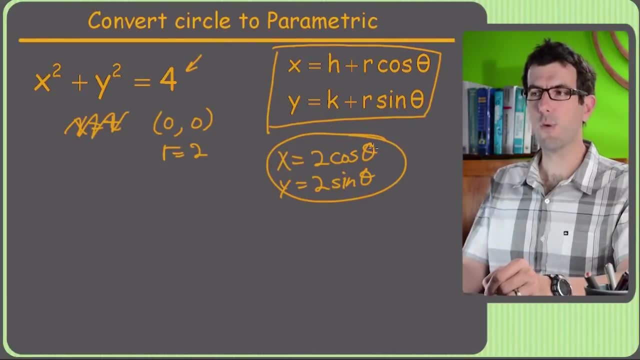 this case plus the radius times cosine theta And y equals the same thing, only sine theta. All right, So it's that easy. If you recognize you're dealing with a circle, just pick out some key information, Plug it into the formula And you're good to go. All right, So that's. 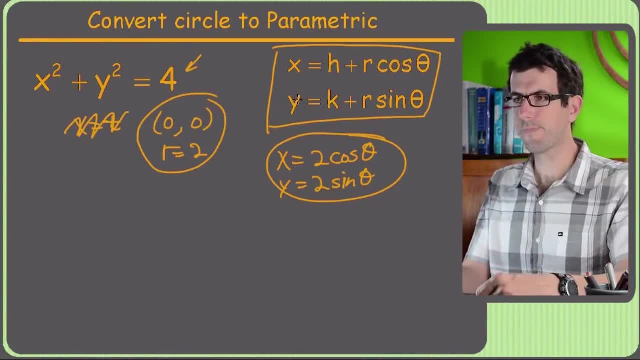 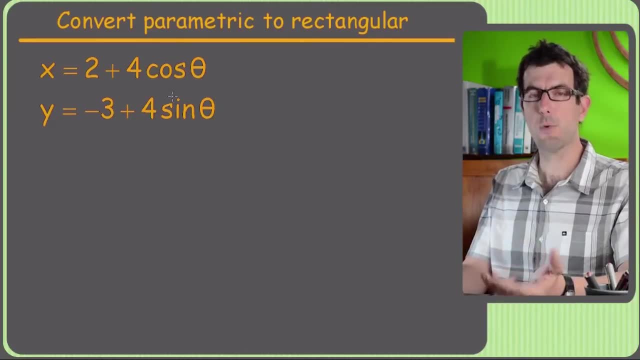 it. So here's the formula as you've memorized, and you're set Going backwards. So here's another circle, only this time it's parametric And we want to convert it to rectangular. So what do we notice right away? How do I know we're dealing with an ellipse or a circle? 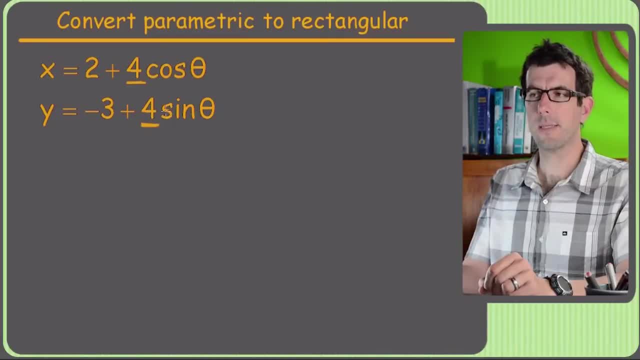 and not an ellipse. It's because the four in both cases. So because the a and the b match, we have the same number in front of both. that means we're dealing with a circle. So what is its radius? Well, r is just the number that's in front of the sine and cosine, So that's a four. 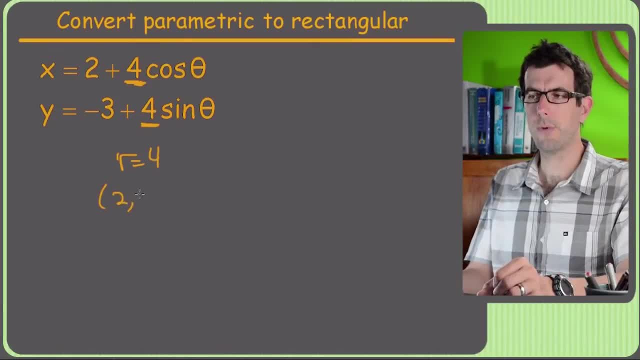 And then the center of this thing is at that coordinate and that other one. So two comma negative three is the center, And we'll just plug and chug through the standard equation of a circle which is x minus h squared, plus y minus k squared, equals r squared, So that 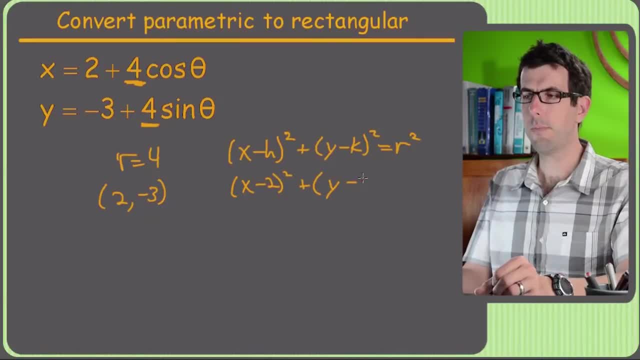 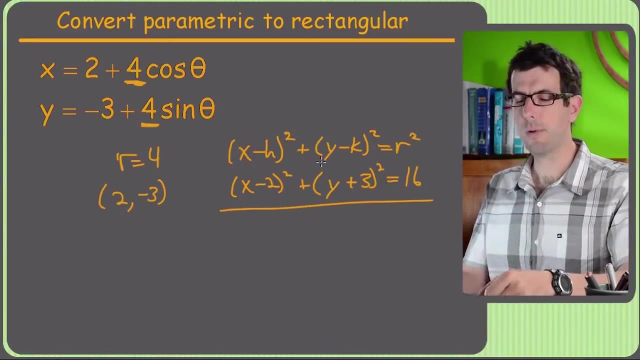 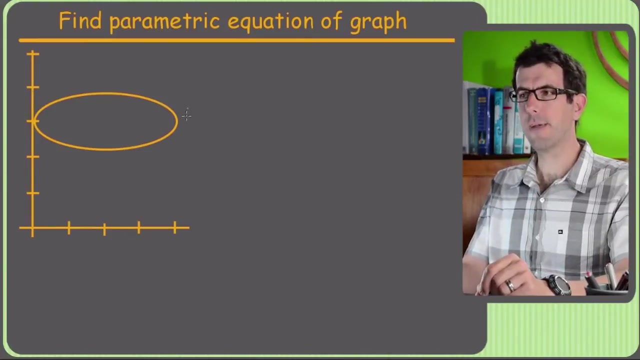 is x minus two squared, y minus the y coordinate, So that's plus three squared, So that's r squared, So that's x minus two squared, So that's plus three squared, So that's two square divided over 16.. 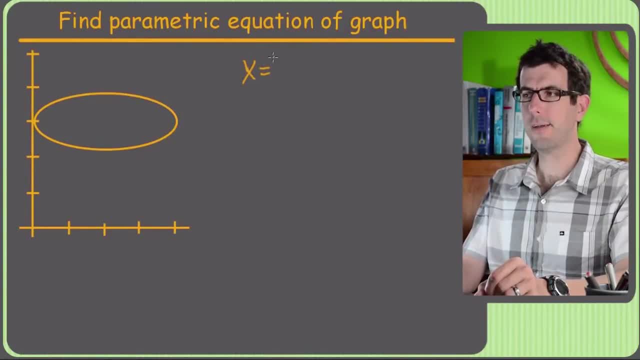 All right, Isn't that wonderful. As long as you spot your equation, pick the key information out, you can just switch willy-nilly between parametric and rectangular. Here's a slightly dicier one. Looks crazy. Here's a graph. It's obviously an ellipse. Anyone wants to find a parametric equation? 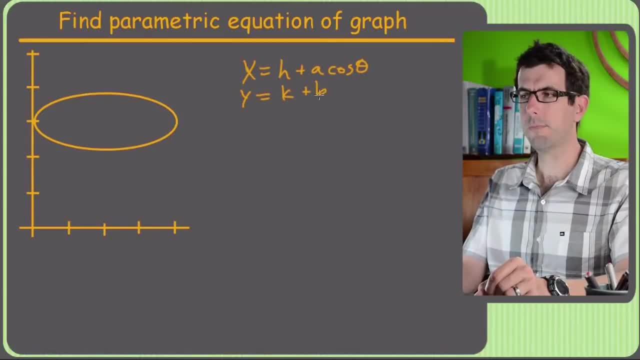 Well. so first in case we don't remember it, x is going to be h plus a cosine data. Well, And y is going to be k plus b cosine theta. So the question is: what's h and k And what's a and b? 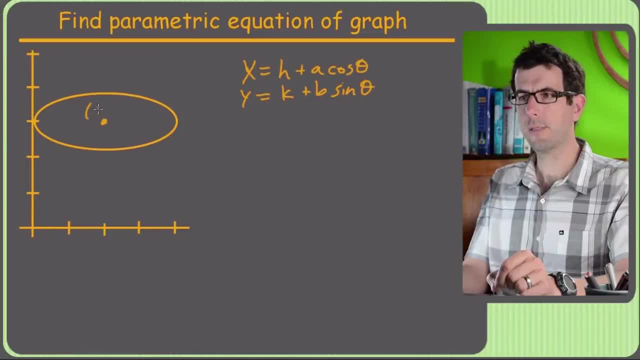 So first of all, let's figure out where the center is. It looks like it's at the point 2, 3.. And then so I've got the center. so h and k. Now the question is, what is a and b? 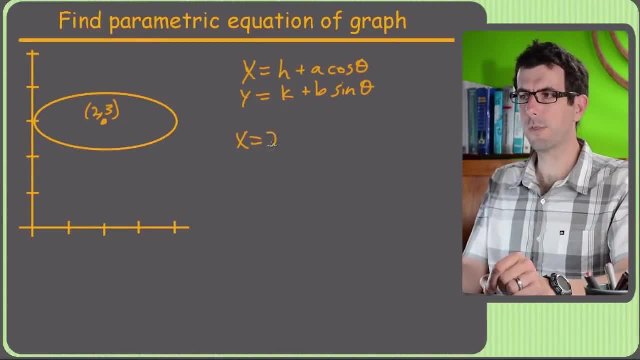 So so far I've got x equals the x coordinate, which is 2, plus something cosine theta, And I've got that y equals 3, the y coordinate plus something sine theta. So now I just need my a and my b and I'll be done. 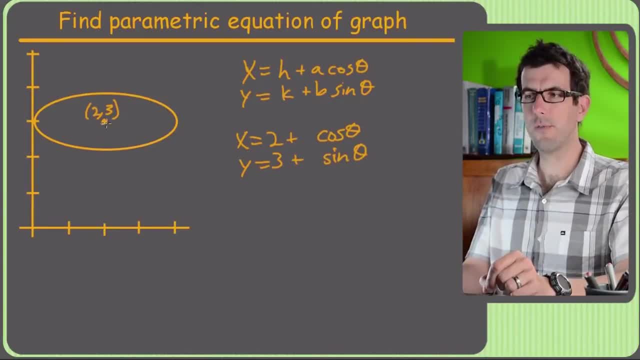 So what goes in front of the cosine in the x equation is just the distance from here to here, And just counting that off it looks like this is x coordinate 2,, this is x coordinate 4, because it's above. x equals 4.. 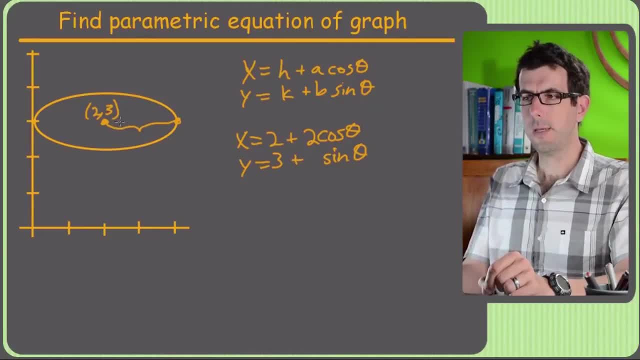 So that little distance is 2, just throw a 2 in there And then this vertical distance is going to be b, from the center down to here, which it looks like is about 1.. So just leave nothing in front of there. an imaginary 1, whatever. 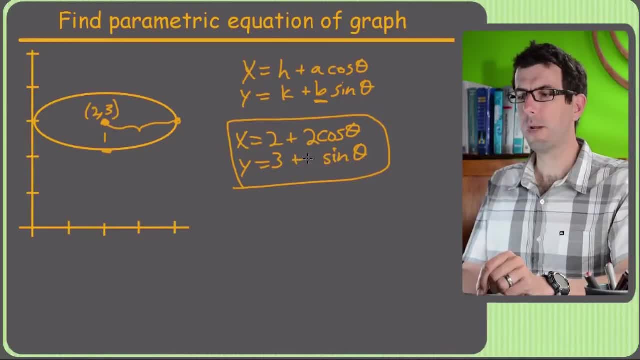 And that is our equation, parametric equation. We could also figure out the rectangular version of this equation And again, if we just go back to the graph, we'll just have x minus the x. So we've got y minus the y coordinate squared, plus y minus the y coordinate squared equals 1.. 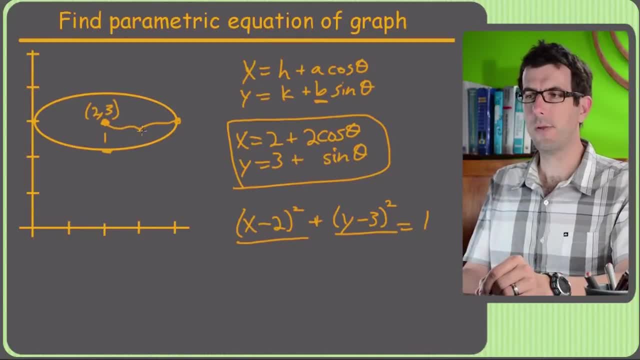 But then the trick is that each one of these is divided by the little a or b squared. So since this was 2 in the x direction, that means I've got a 2 squared down here, And since this dimension is 1, I've got a 1 squared right there. 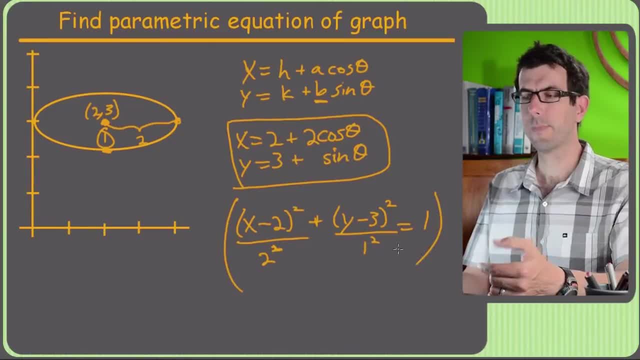 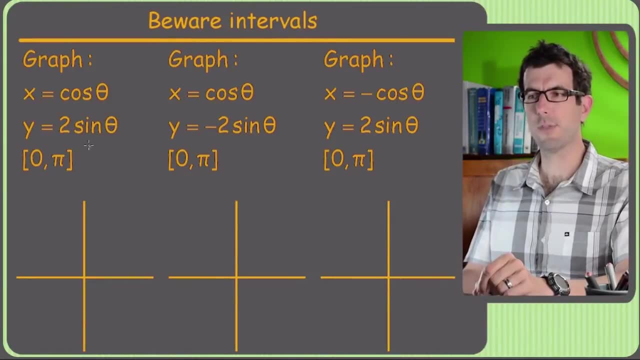 That would be the standard rectangular version of an ellipse. All right, beware intervals. So what we mean by intervals is that they gave us a limitation. It's just from 0 to pi. Now, what I've done here is I've given us the same three equations. 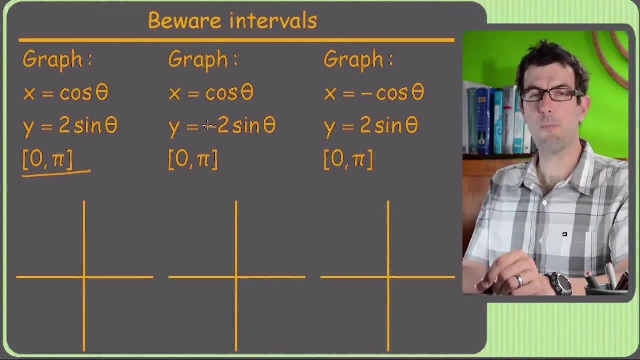 and I've just put some different negative signs in, because that actually will mess with you in a parametric equation. So let's take a look Now. just by looking at it, it seems that we have an ellipse, because in all three of these pairs of equations, 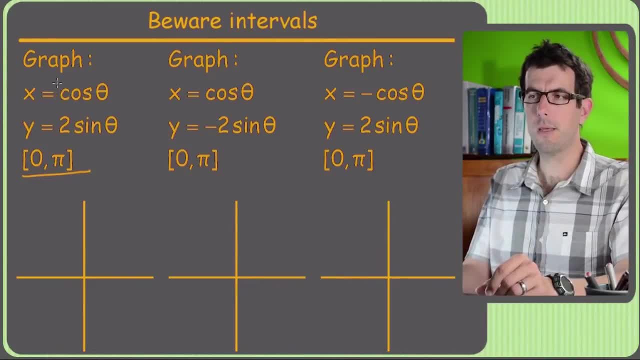 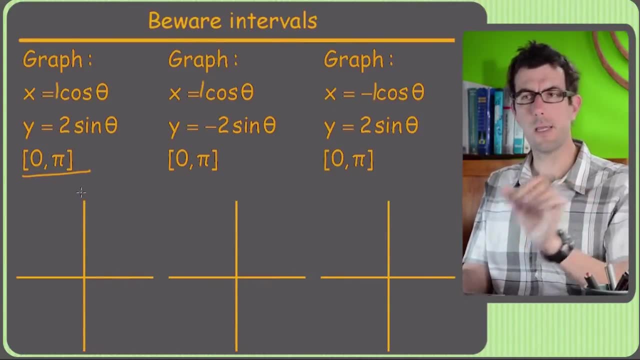 we've got a cosine and sine, just like usual, except we've got a 1 in front of the cosines And we've got a 2 in front of the sines. So that means we have a tall and skinny ellipse. 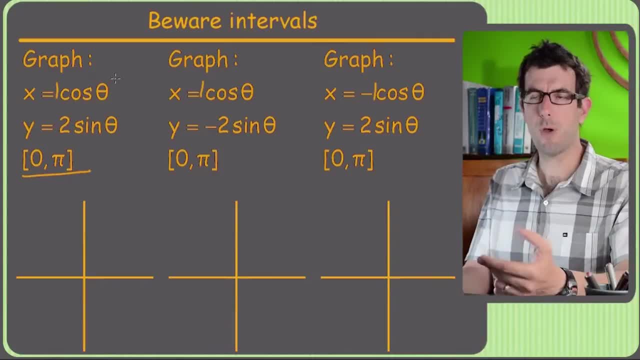 So the x coordinates, and you can kind of see that since cosine goes from negative 1 to 1, our x coordinate is going to go from negative 1 to 1, but our y coordinate is going to go from negative 2 to 2,. 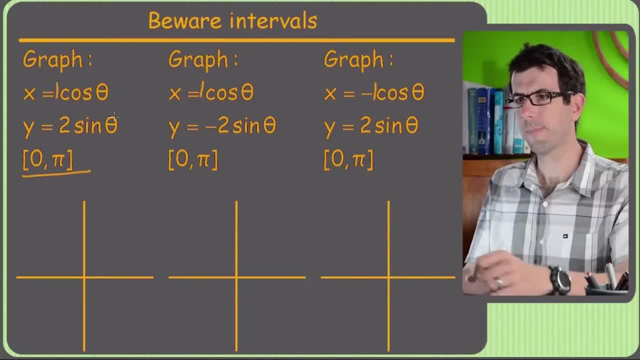 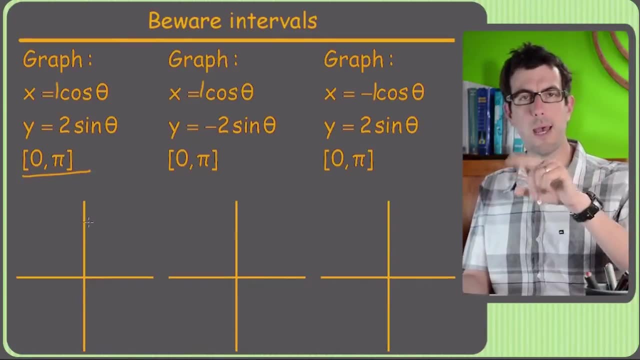 because there's sort of like an amplitude of 2 in front of the sine. So the question is what happens as we go from 0 to pi? Do we get the top half of the ellipse, the right half, the left half? 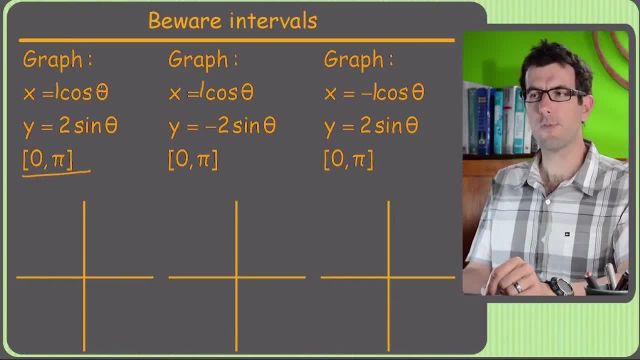 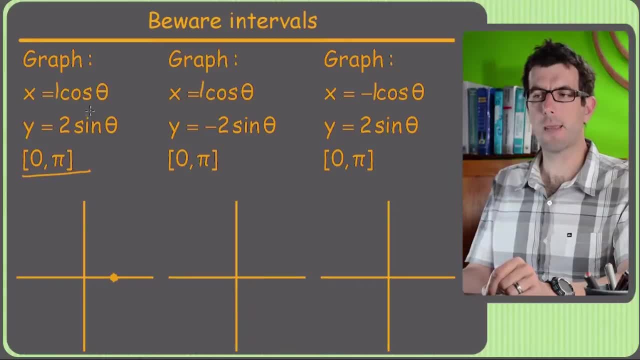 Then if you plug in pi, you'd get negative 1, 0. And the question is: do we go up over the top to get to there or do we go underneath? And it looks like, if we plug in pi over 2, which is halfway through the interval. 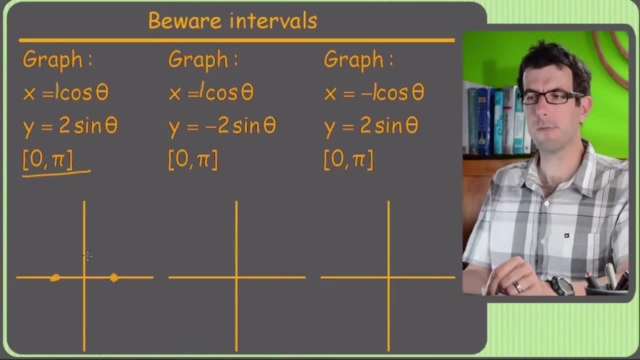 we'll get positive coordinates And we'll get a positive 0,, 2.. So we'll get through this point. So the graph, So the graph of the parametric ellipse, it's just the top half and it's going this direction. 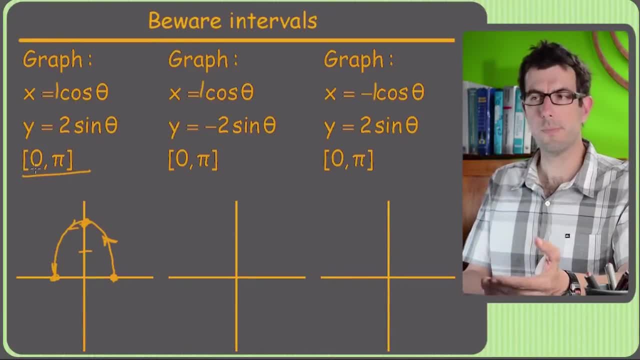 Because as we go from smaller, you know, from 0 to pi, so going from smaller numbers to bigger numbers, we work our way counterclockwise around that semi-ellipse, that half-ellipse. So what's going to happen to this one? 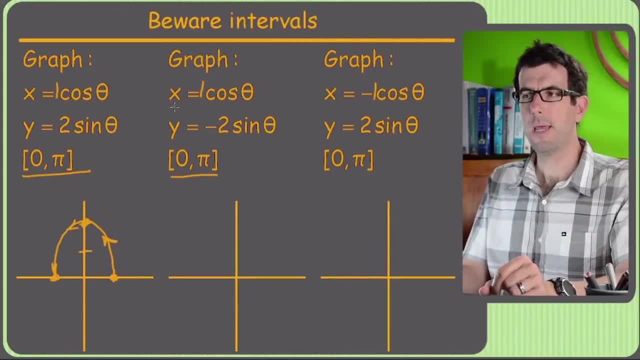 Looks like my x-coordinate. So once again we have the same interval, 0 to pi, And my x-equation is exactly the same as last time. So my x's should go. If I plug in 0,, I'll get 1.. 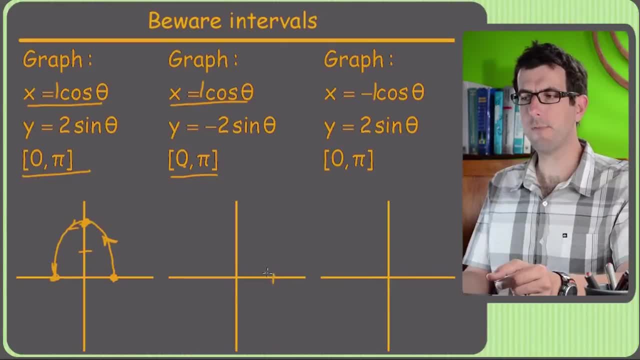 If I plug in, If I plug in pi, I'll get negative 1.. So x is going to go from positive 1 to negative 1.. But look at this: negative 2.. Sine, that's just going to basically flip this thing over. 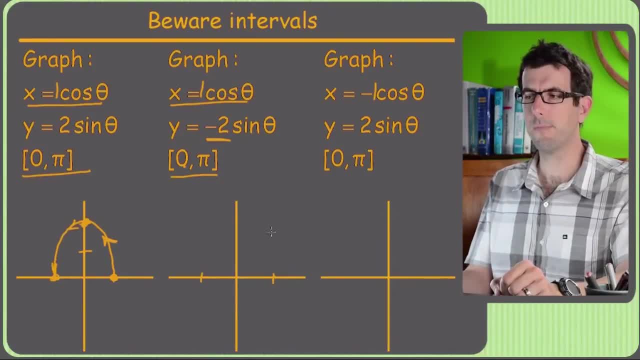 We're just going to reflect it like this. If you wanted to, you could plug and chug, though. So we'll get from this point to this point If we plug in pi over 2, right in the middle of the interval. 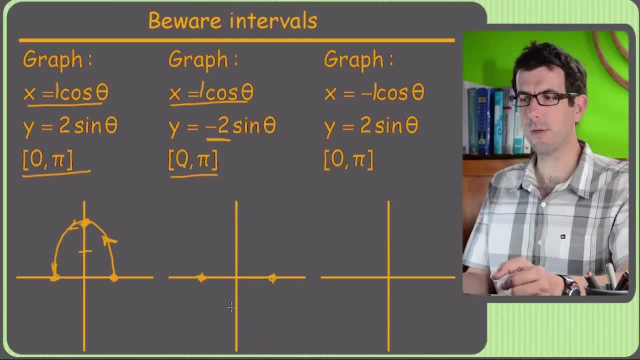 sine of pi over 2 is 1, but multiplied by negative 2, we get negative 2.. So this point is in the arch. So the graph looks like it's a semi-ellipse. again, This time it's going that way. 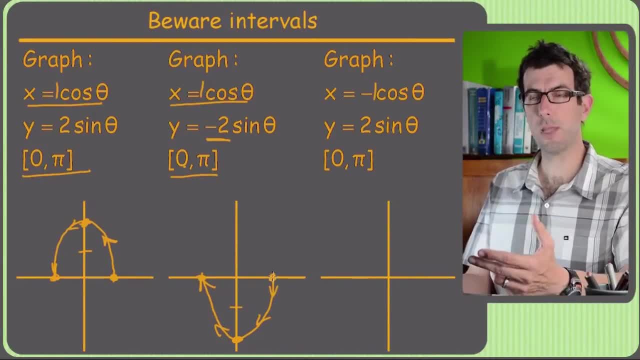 Since we're going from Again, we're going to go in the direction. as we plug in the parameter, It gets bigger and bigger. So if we start at 0, that's our starting point, Our ending point is at pi, which is right here. 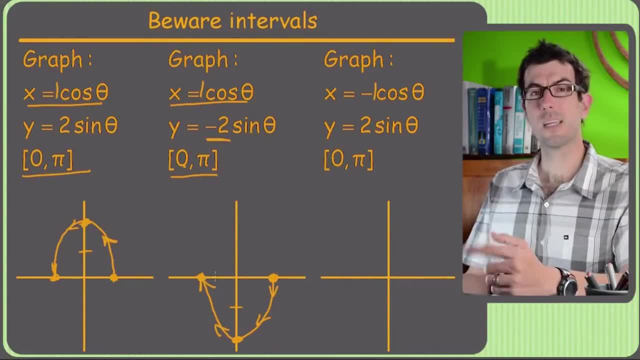 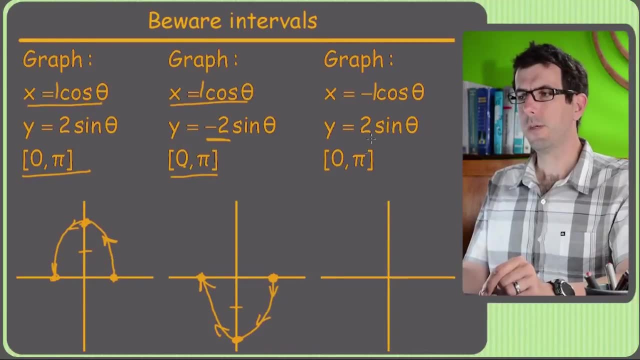 And as we work our way along the interval, we work our way around the ellipse clockwise, this time semi-ellipse. All right, and this last one, we throw a negative in front of the cosine data. So that means our starting point. when you plug in 0, you get negative. 1 for x. 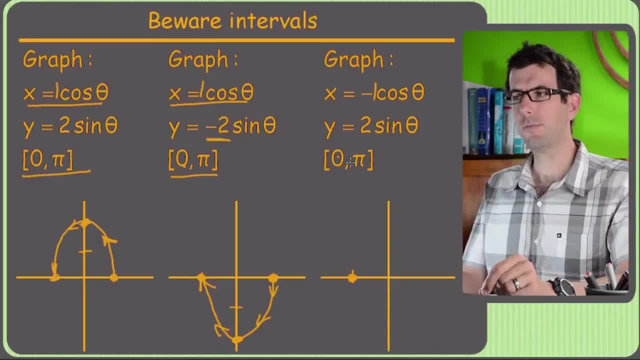 0 for y. Then when you plug in pi over 2, you get 0 for x and positive 2 for y, And then when you plug in pi, you get negative, negative 1, which is positive 1, comma 0.. 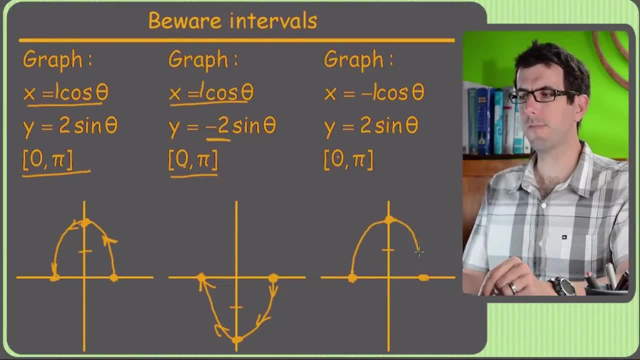 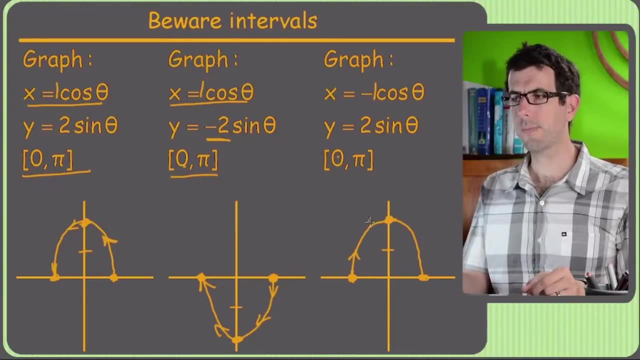 So this time we get a graph that looks identical to the first one, except instead of the arrows going like this, they're going to go the other way. Okay, So we're going to go here and go this way along the curve. 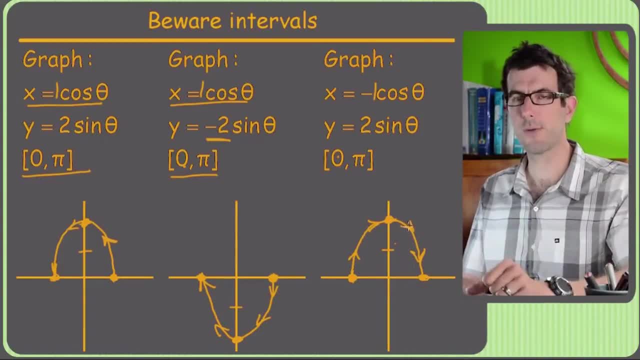 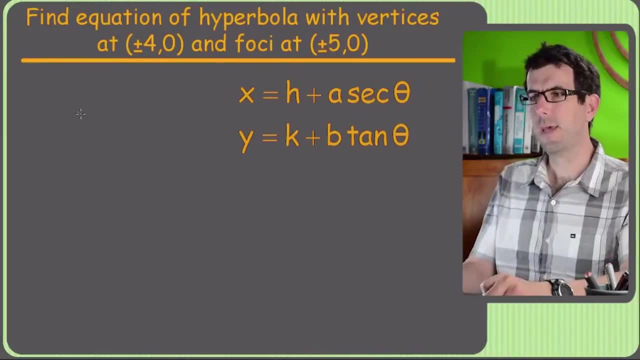 And, like I said before, if you have one of those teachers who's a stickler for these little direction arrows, you don't want to leave those off. That's the direction of the path. if your teacher's into calling these paths, All right. and the last one we'll do here is a quick hyperbola. 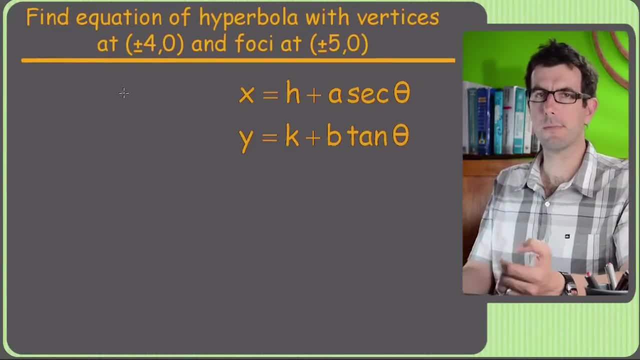 But, like I said, these aren't super common. Most teachers don't do them because it's- I don't know, just kind of pointless. All right, so find the equation of the hyperbola, and I've given you the vertices. 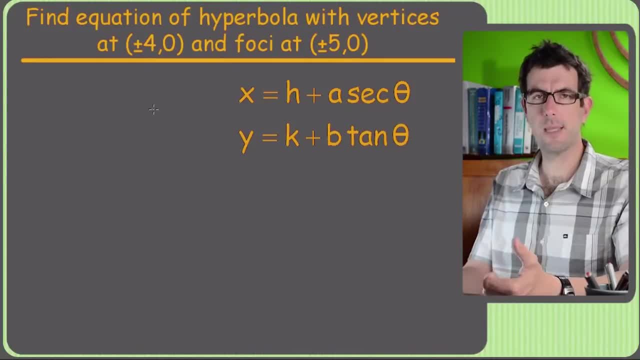 Now, this is not the easiest problem. I could have asked. We could have said: hey, you know, given you its center, given you its width and height and stuff, it's A and B, because you'll notice, we have an A and B here. 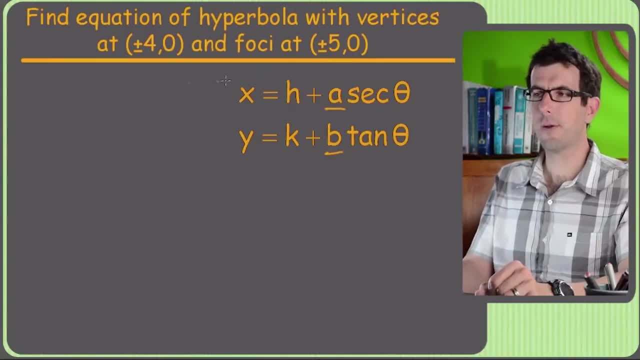 But what do we do with a foci? What's that? Well, just as a reminder, a hyperbola, that's the one where you kind of like drew a box and then put asymptotes like this, and then the hyperbola was like this: 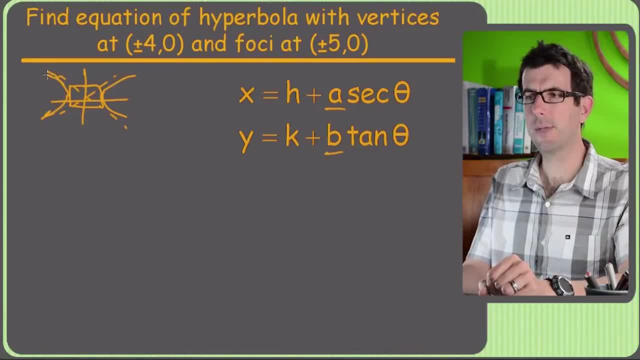 Kind of had two mirror halves. If you don't remember that, and your teacher's one of these ones doing hyperbolas, you probably won. So you might want to go back and watch the Algebra 2 chapter on conics and just remind yourself. refresh yourself on the hyperbolas. 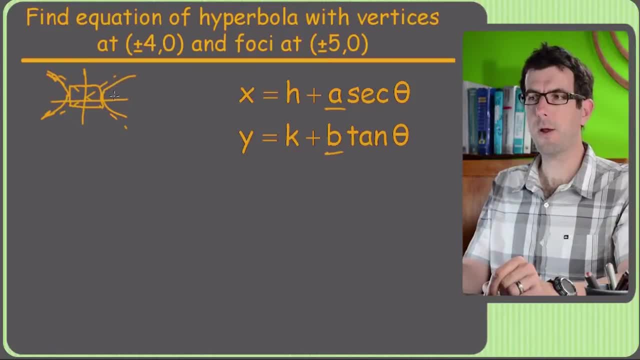 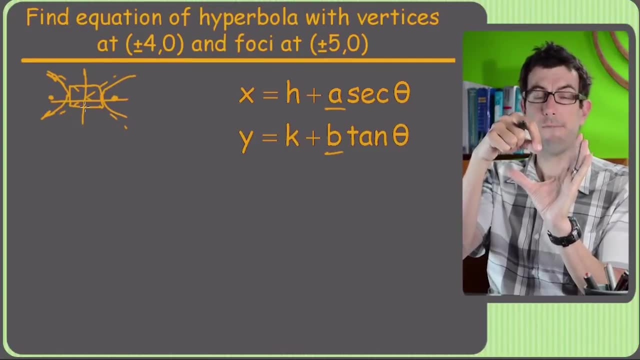 But the point is that these foci in a hyperbola are out here. They're kind of like in a satellite dish or something. You've got that little antenna sort of sitting right above the dish. That's the focus of the satellite dish and that's what these are. 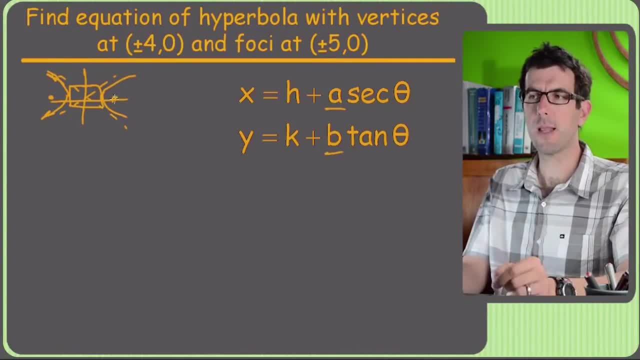 So I just always the way I remember where the foci are of a conic is they're kind of like inside the curve, You know if they're inside an ellipse, but they're on the outside of a hyperbola. 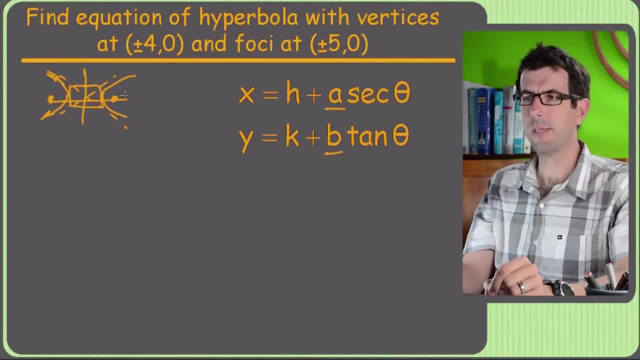 So they're out here. So they've just given us the coordinates that these are at the point five comma zero and negative five comma zero, But then the vertices, which is right here- those are at four comma zero. So the question is: what are A and B? 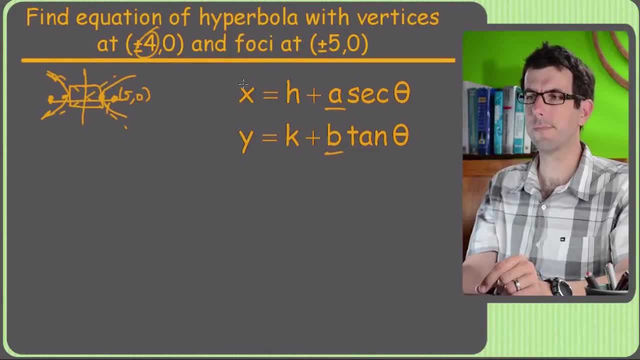 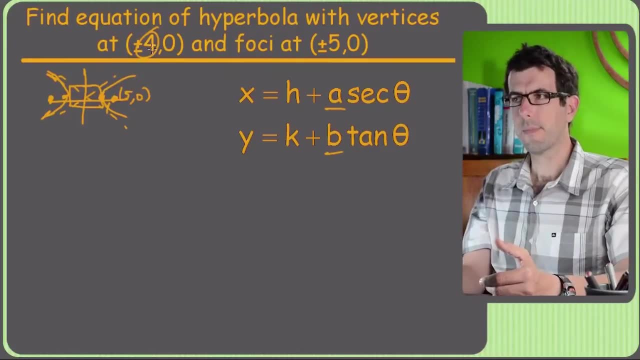 Well, it turns out that this distance right here, that's A, So right away, and we know this thing is centered at zero because these foci and the vertices are both symmetrical about the origin, So it looks like the center of this thing is right at the origin. 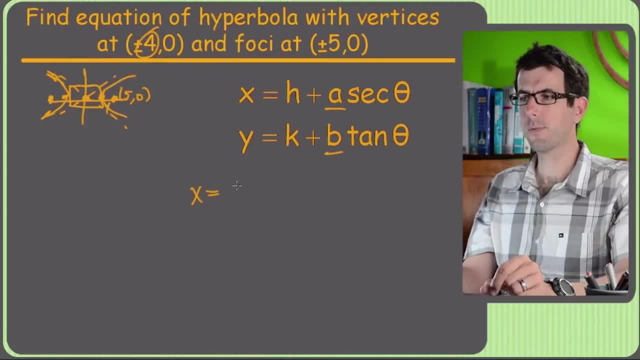 So that means I can just start plugging and chugging. X equals zero plus something secant theta, and Y equals zero plus something tan theta, Now A, because there's a horizontal distance that they've given me to four comma zero. 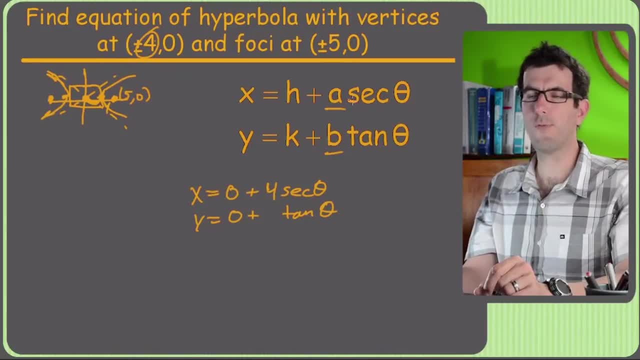 this distance right here is four, So that means we have our A is four, Our little X, Our X coordinate, our X stretch is four, So that goes in the X coordinate, the X equation right there. The question is: what's the Y coordinate? 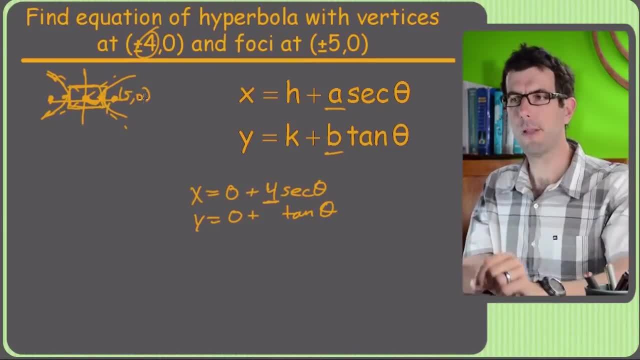 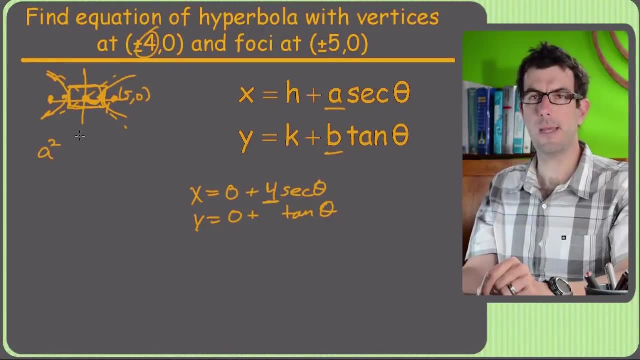 How tall is this little box? you know, to give me the parabola, the hyperbola, Sorry. So it turns out. we have to figure that out with a little equation. And again, you may recall this, you might not. 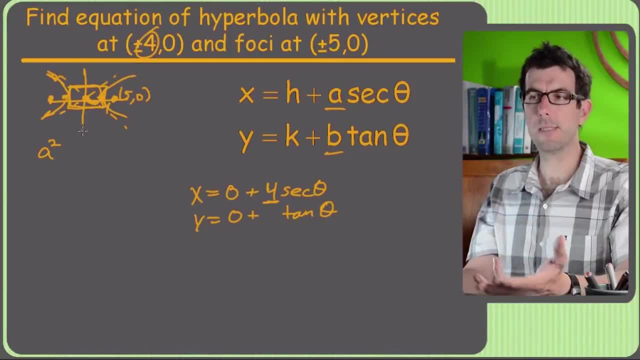 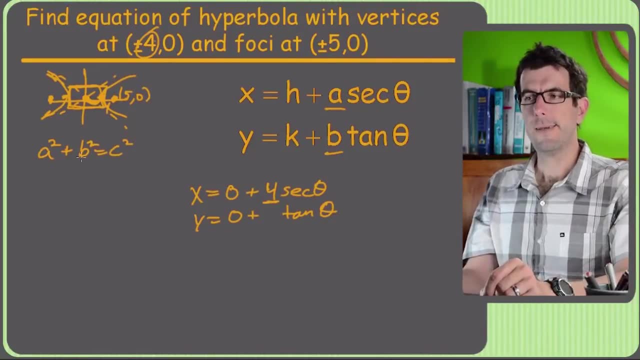 But in all these conics there was always a relationship between A, B and C And it was: in hyperbolas it's A squared plus B squared equals C squared. In ellipses it was opposite. So it was more like B squared equals A squared plus C squared, or something. 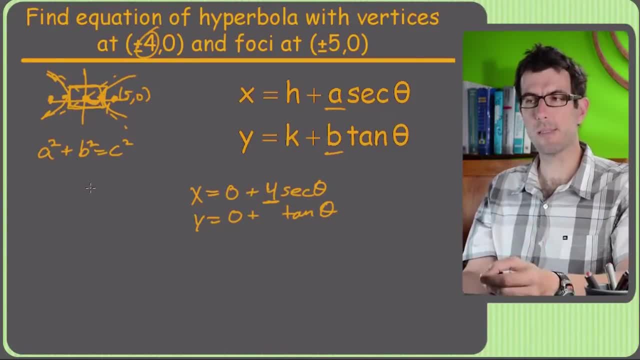 The way I remember it is. I just look at the graph, look at whichever one's biggest and put it by itself on one side. So, since the foci are way outside that graph, they're bigger than A and they're probably bigger than B. 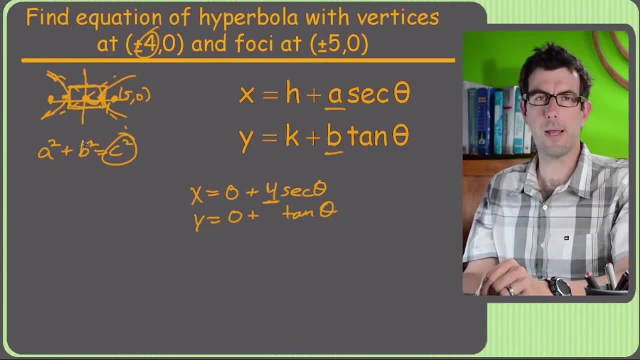 So that's how I know C squared goes by itself, And then the other two squared added up on the other side. But the point is we got A squared plus B squared equals C squared, Since I know C is five and I know A was four. 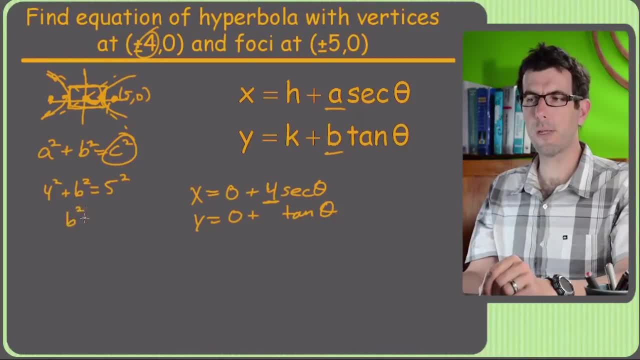 I can solve pretty quick to get that B squared equals 25 minus 16, which is nine. so B equals three And that's how I get a three right here. But again, if you have one of these teachers, who's actually going to do hyperbolas? 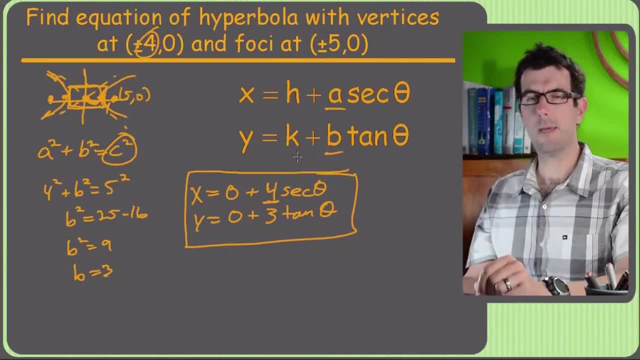 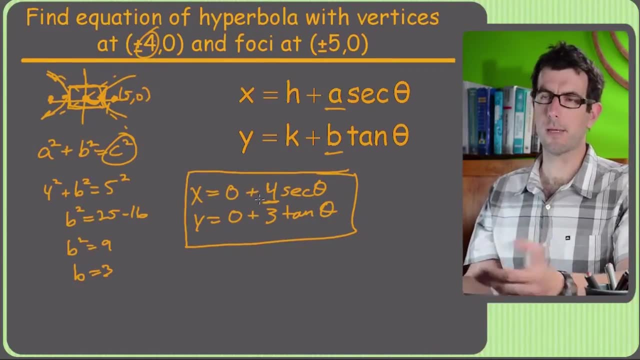 in parametric formula form, then you're just going to need to practice this a little bit. But, honestly, even if you had that teacher, it's probably going to be more about ellipses and circles anyway, because they're a little bit more varied, a little bit more fun. 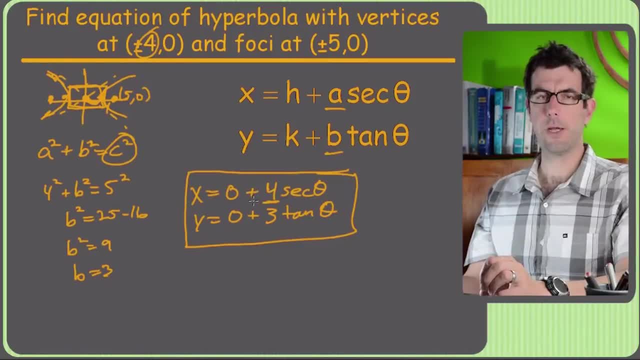 So there you go, Live it up, love your parametric equations, But know that this stuff is kind of pointless. It'll come and go this one time. The exception is projectile motion, So I'm actually going to make that a separate chapter about projectile motion.